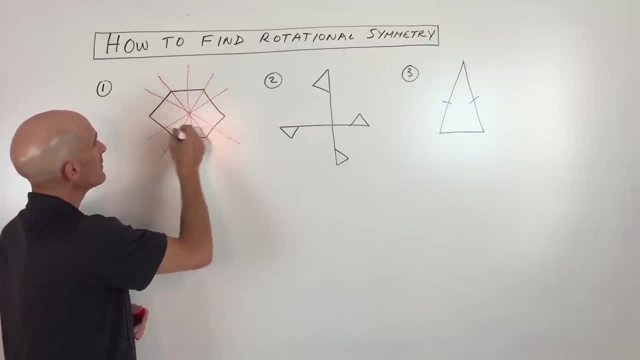 So that would be four, five and six. So there's six lines of symmetry. If we take 360 degrees divided by the six lines of symmetry, you can see we're getting 60 degrees. So what that means is that if we rotate about this point 60 degrees, it's just like a knob. this object will match up. 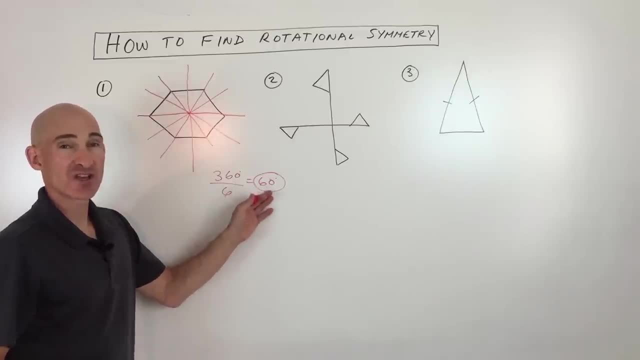 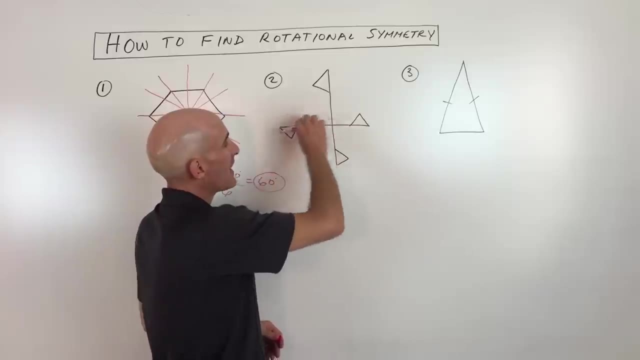 with itself. So we can say this has 60 degree rotational symmetry. Okay, example number two: When we look at this figure here, there aren't any lines of symmetry, Like if I draw this, like this, let's say on this angle, like here if I fold it. 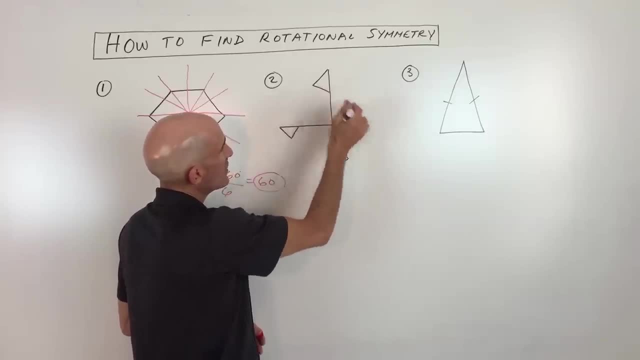 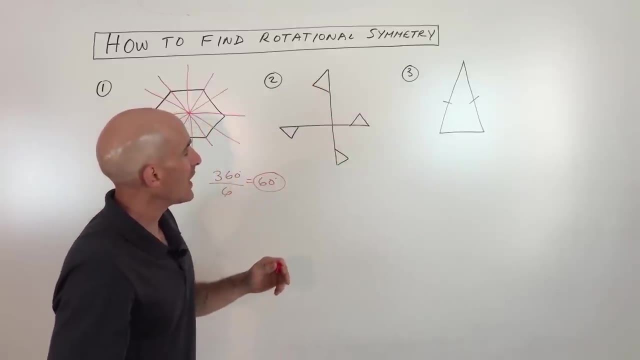 over. it doesn't actually match with this figure here. It's, you know, it's. it doesn't match up perfectly. I guess the only way I can say it. when you fold it, this is going to be pointing in a slightly different direction, And so this one it's, maybe not. we can't really solve it the way we did. 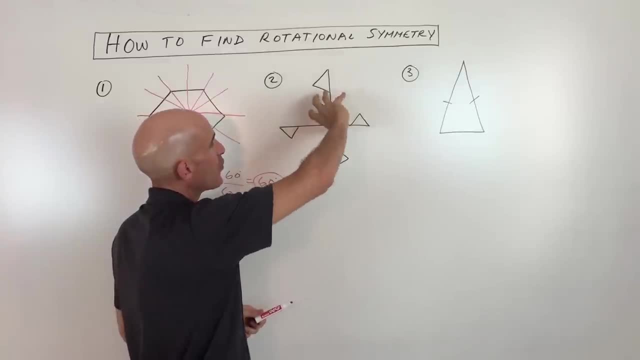 this one. but you can still see that if you were to take this object and turn it around, it would turn it a quarter, turn 90 degrees, that this, you know- flag or triangle is going to then match up with this one, this one's going to match up with this one, and so on. And so by doing it 90 degree, 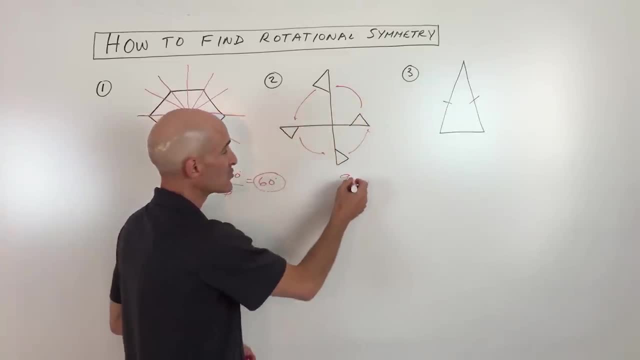 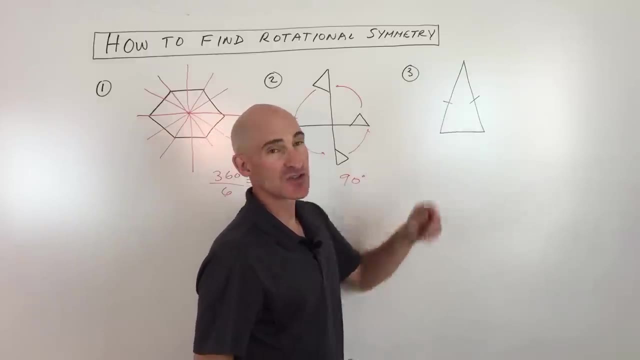 turn or rotation, this will match to itself. So this does have rotational symmetry: 90 degrees, Okay, third example: Here I've drawn a triangle for us, an isosceles triangle, and you can see that there's a line of symmetry that goes right down the middle, like so Meaning if we fold it over. 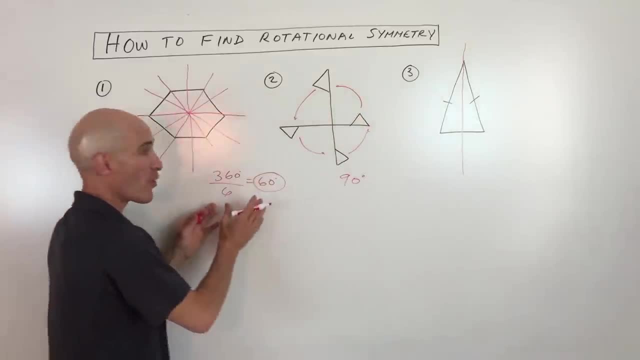 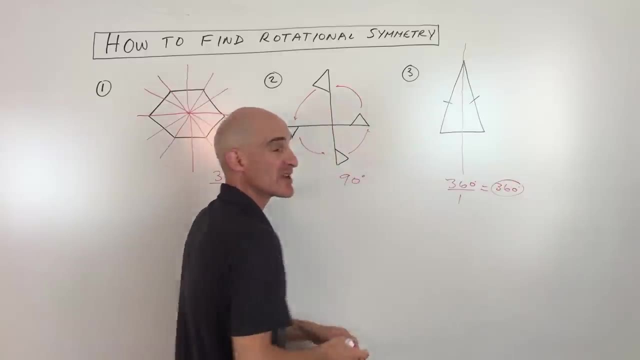 this line, it's going to match to itself. So in this one where we took 360 degrees and we divided it by the number of lines of symmetry, you can see we're just getting 360 degrees. Well, 360 degrees if you take any object and you turn it all the way. 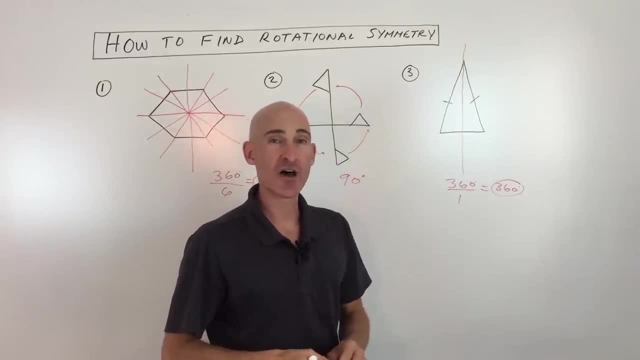 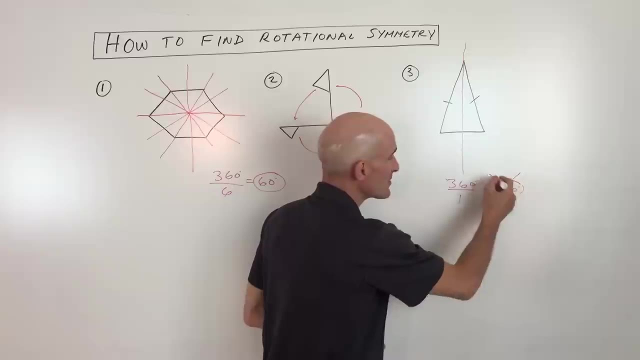 around. okay, a full turn, and actually it will match with itself. okay, because you've done a complete revolution. it's in the same position it was in originally, so we don't consider this having any rotational symmetry. 360 doesn't count. It's going to be anything between 0 and 180. okay, It won't.